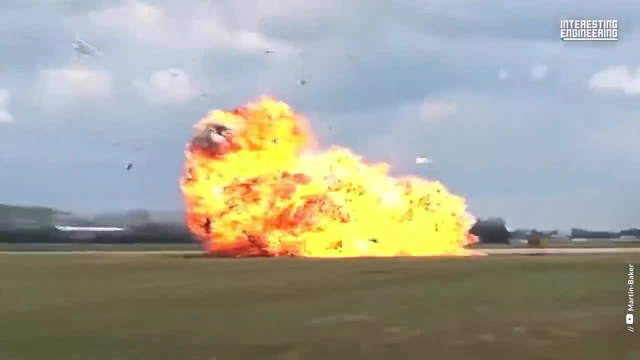 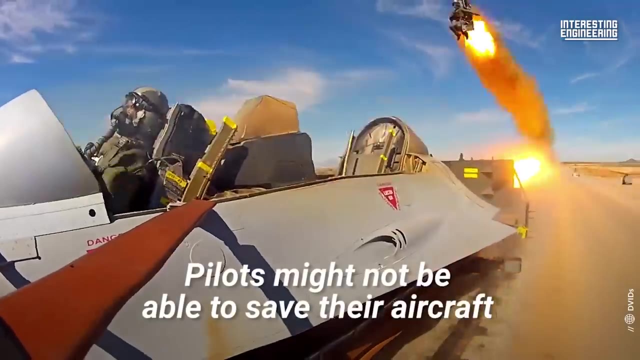 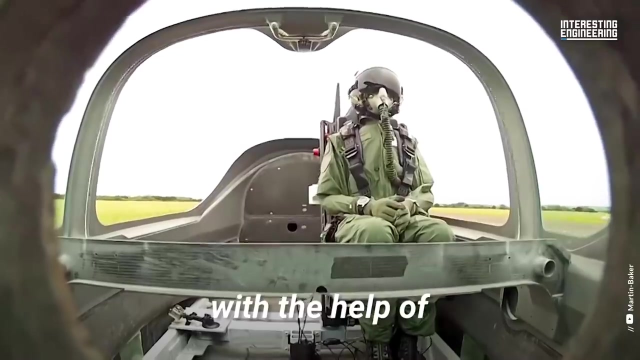 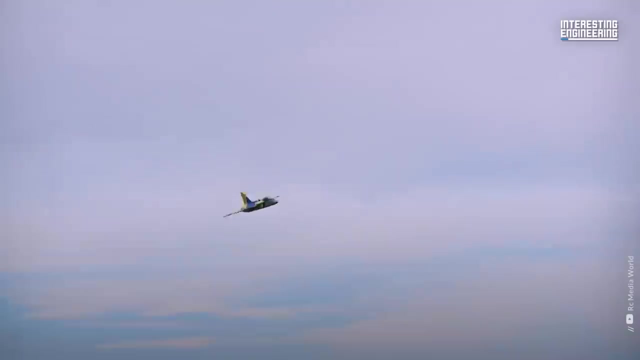 Even the best fighter jets in the world could fail. Pilots might not be able to save their aircraft, but they could safely exit a fighter jet and avoid certain death with the help of ejection seats. Here's how they work. Seats are called mayday and are lifted straight out of the crashing aircraft. 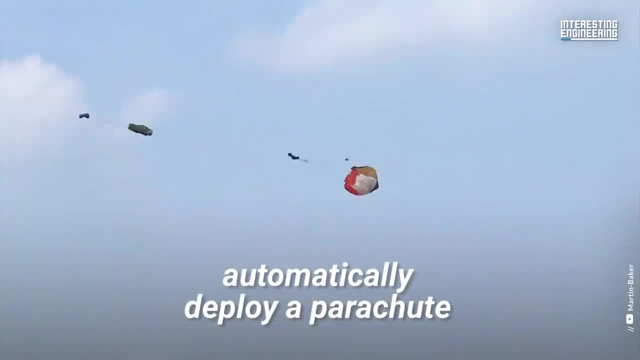 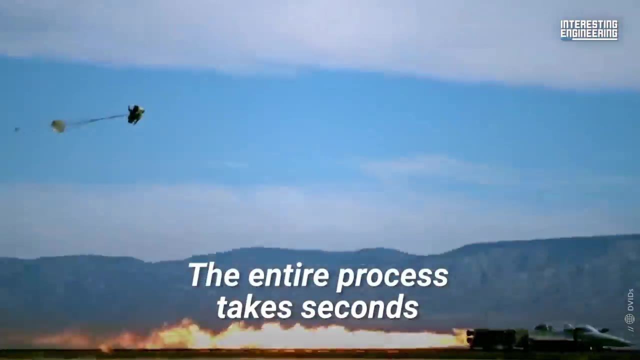 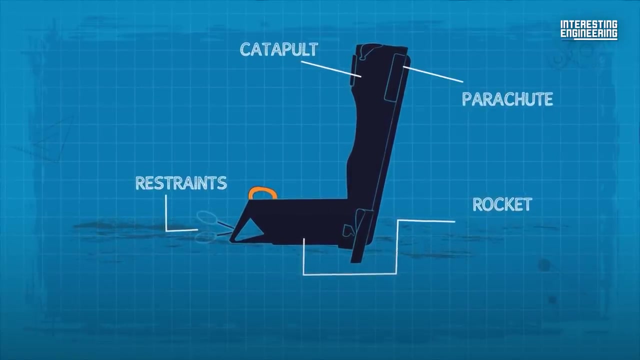 Once the coast is clear, ejection seats then automatically deploy a parachute allowing pilots to descend safely. The entire process takes seconds. The main components of an ejection seat- the catapult, rocket, restraint and parachute- all have to trigger in a certain sequence and near instantly. 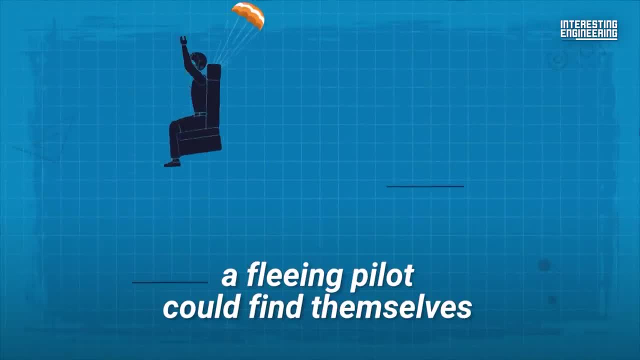 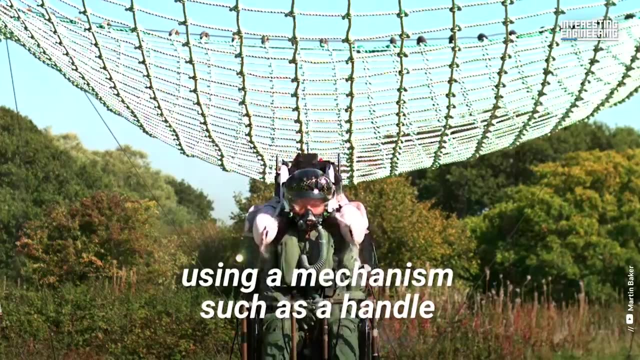 If even one step goes awry, a fleeing pilot could find themselves in a whole lot of trouble. Once a crew member triggers the ejection process using a mechanism such as a handle, they'll be out of the plane in less than a second. 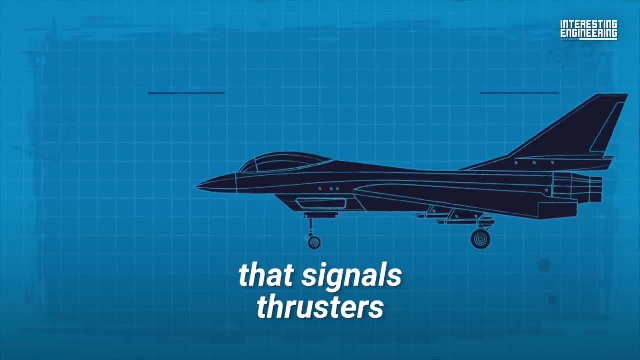 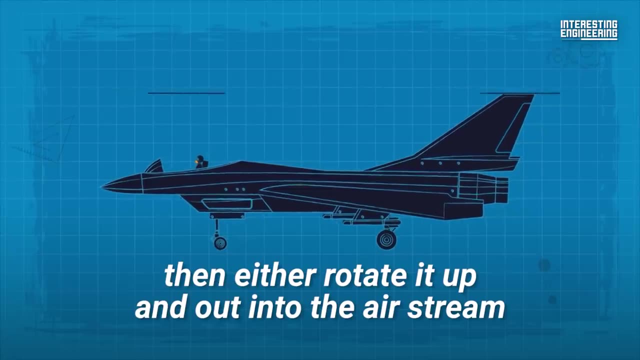 Pulling on the ejection handle sends an electrical pulse that signals thrusters to blow the canopy or unlock the hatch, then either rotate it up and out into the airstream or blow it out of the plane. At almost the same time, an explosive current is released from the ejection seat. 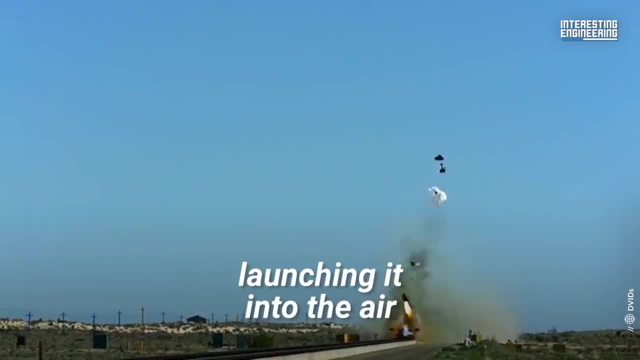 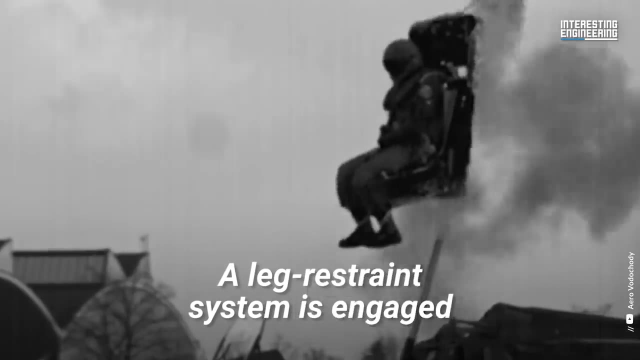 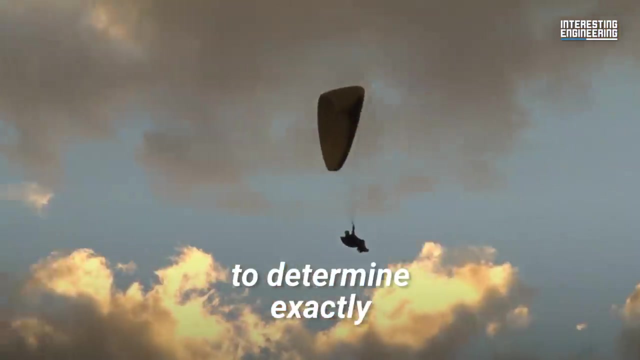 A cartridge is set off in the seat's catapult gun, launching it into the air with the help of an under-seat rocket motor. A leg restraint system is engaged to protect their legs from debris. Sensors measure the speed of the airplane and ambient air pressure to determine exactly. 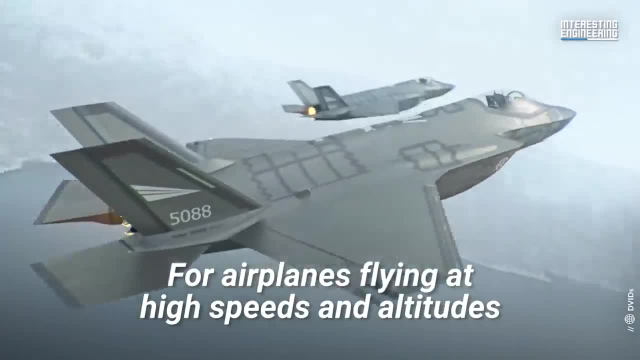 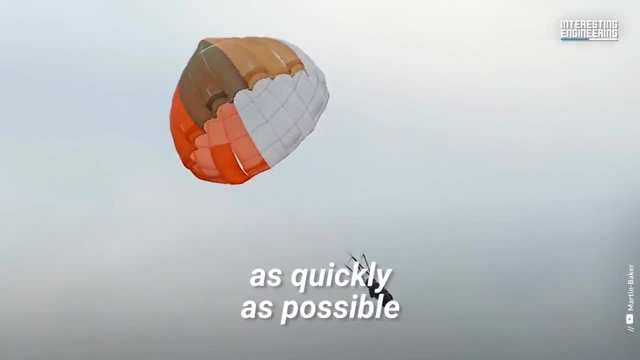 when to deploy the parachute. For airplanes flying at high speeds and altitudes, the opening of the main parachute is delayed to get the pilot down to thicker air as quickly as possible. The ejection system is designed to allow the pilot to fly at high speeds and altitudes. 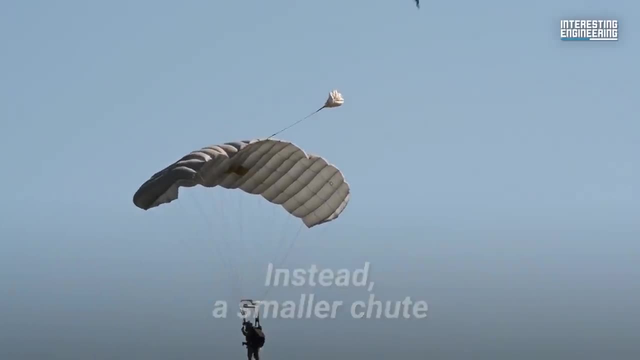 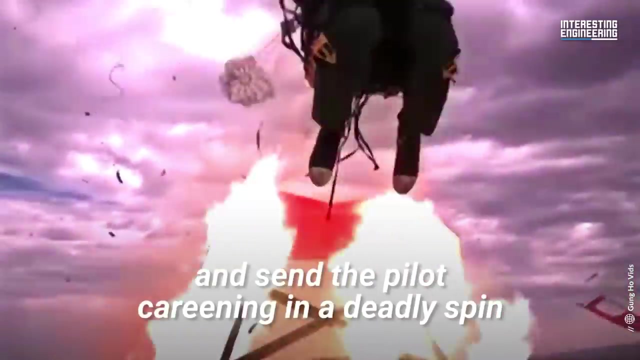 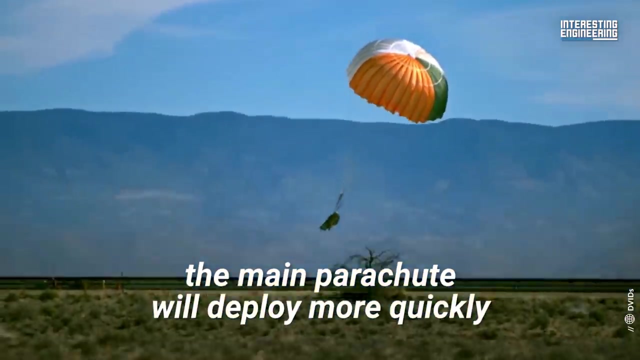 Instead, a smaller chute called a drogue deploys to slow down the rate of descent and stabilize the motion so it doesn't tumble and send the pilot careening in a deadly spin. At lower speeds and altitudes the main parachute will deploy more quickly.